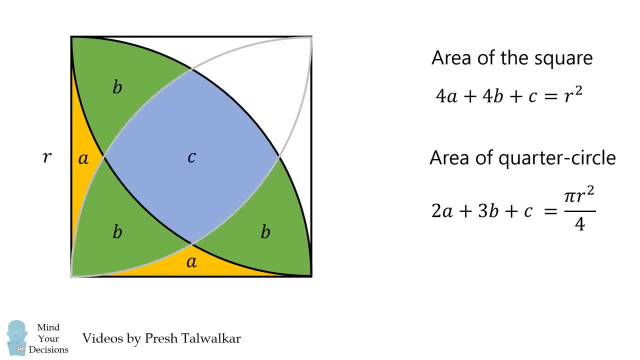 It'll also be equal to 2a plus 3b plus c. We now have two equations for three variables. Let's get a third equation. We'll calculate the area of this shape here. To do that, we'll do some preliminary work. 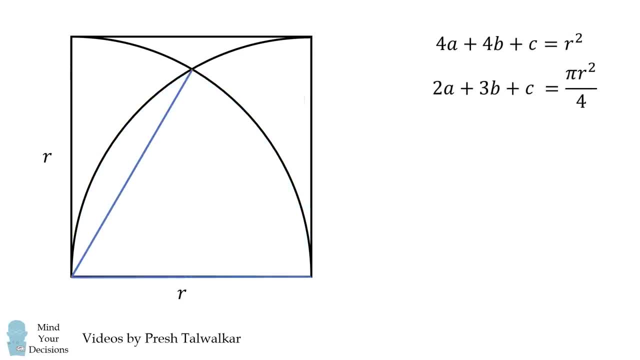 The side of the square is equal to the area of the square. The side of the square is equal to r, and that means the radius of this quarter circle is equal to r and the radius of the other quarter circle is also equal to r. 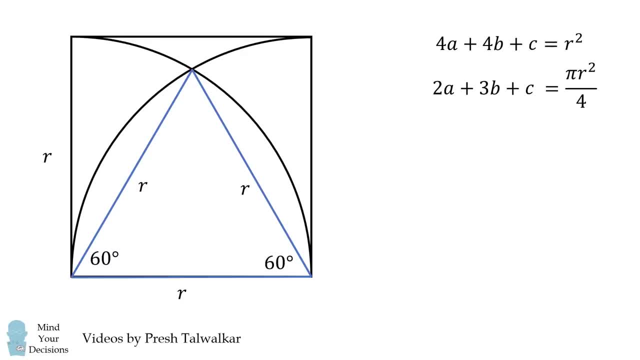 We have an equilateral triangle, so each of its angles is equal to 60 degrees. Let's calculate the area of this circular sector. It'll be equal to pi r squared multiplied by 60 degrees over 360 degrees. This simplifies to be pi r squared over 6.. 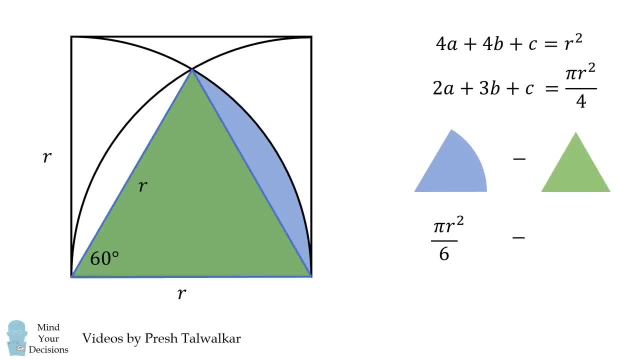 We can then calculate the area of this equilateral triangle, which will be r squared over 6.. If we subtract the equilateral triangle's area from this circular sector, we get the area of the circular segment. If we flip this circular segment horizontally, 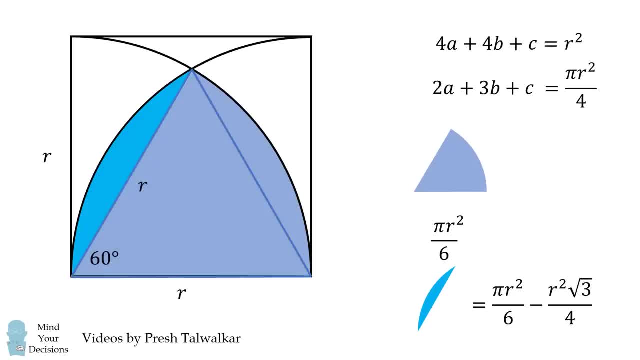 we get the other one on the other side of the triangle, We'll add this area to the circular sector and we get the area of the shape that we want. We'll simplify this formula a little bit and then we'll go back to our a, b and c diagram. 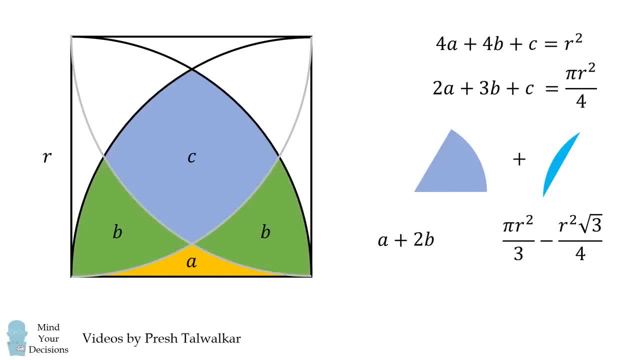 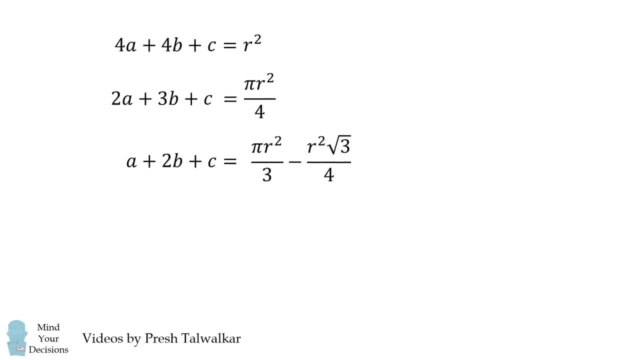 so we get that the area is equal to a plus 2b plus c. We now have three equations for three variables and we can very carefully solve for a, b and c. First we'll eliminate c by subtracting the second equation from the first equation. 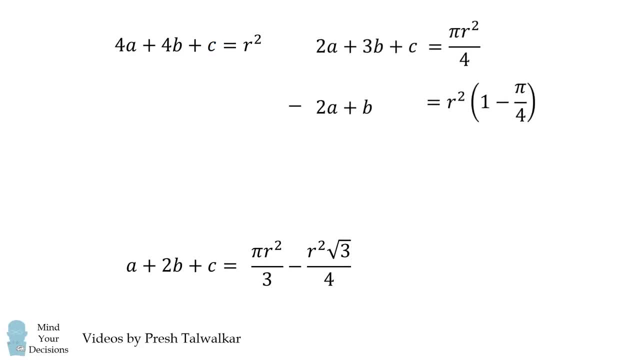 Then we'll eliminate 2a by doing the following subtraction: We end up that 2b plus c is equal to the following, which we'll substitute in to this last equation. This is an equation only in a, so we'll solve for the variable a. 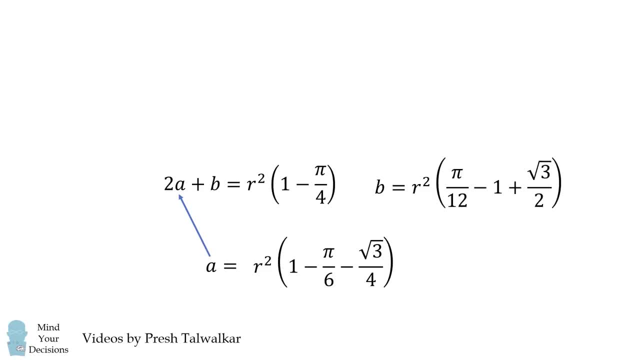 Knowing the value of a, we can substitute back and get the value of b. Knowing b, we can substitute back and get the value of c, And there you go. this is the solution to our problem. We've calculated the areas of a, b and c using only geometry and a little bit of algebra. 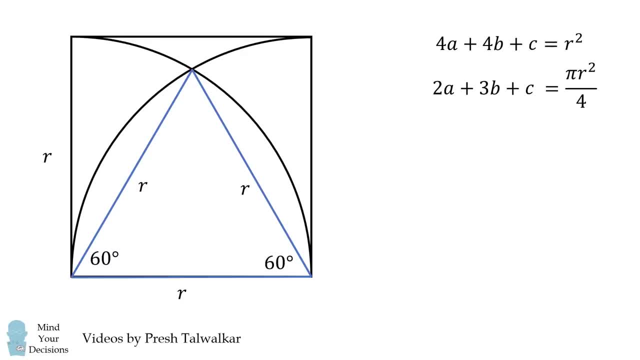 We have an equilateral triangle, so each of its angles is equal to 60 degrees. Let's calculate the area of this circular sector. It'll be equal to pi r squared multiplied by 60 degrees over 360 degrees. This simplifies to be pi r squared over 6.. 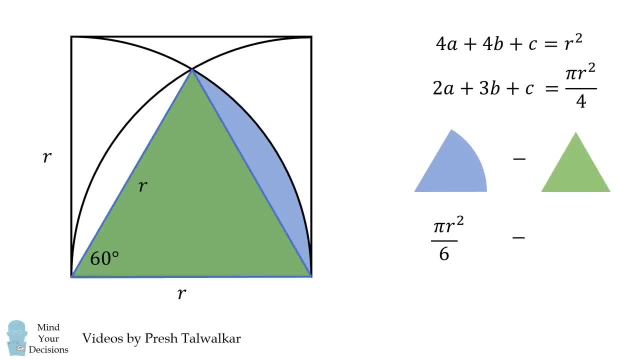 We can then calculate the area of this equilateral triangle, which will be r squared over 6.. If we subtract the equilateral triangle's area from this circular sector, we get the area of the circular segment. If we flip this circular segment horizontally, 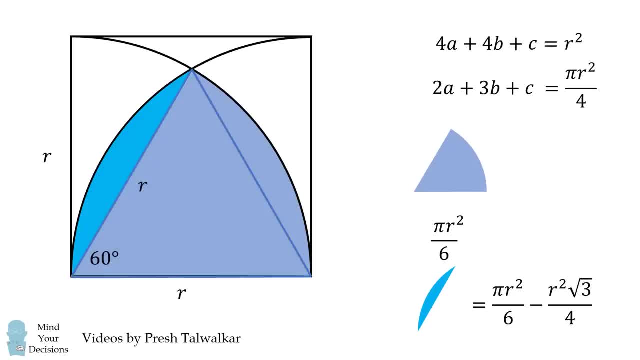 we get the other one on the other side of the triangle, We'll add this area to the circular sector and we get the area of the shape that we want. We'll simplify this formula a little bit and then we'll go back to our a, b and c diagram. 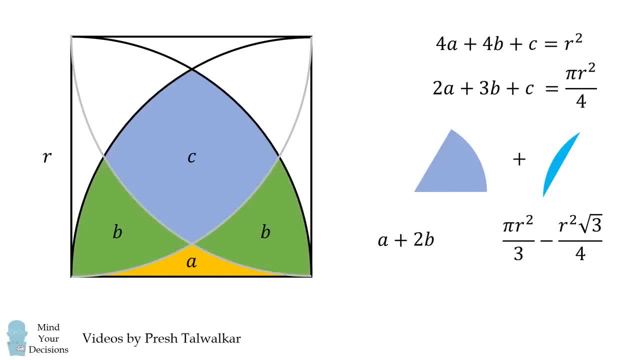 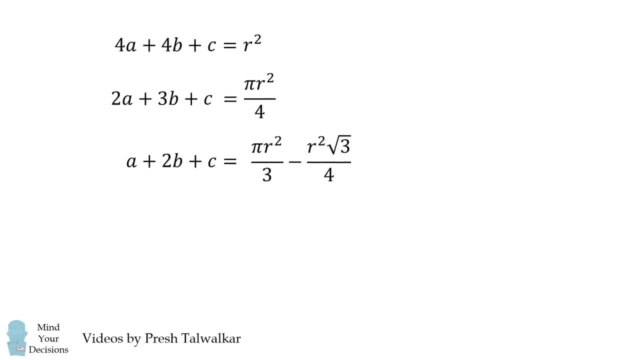 so we get that the area is equal to a plus 2b plus c. We now have three equations for three variables and we can very carefully solve for a, b and c. First we'll eliminate c by subtracting the second equation from the first equation. 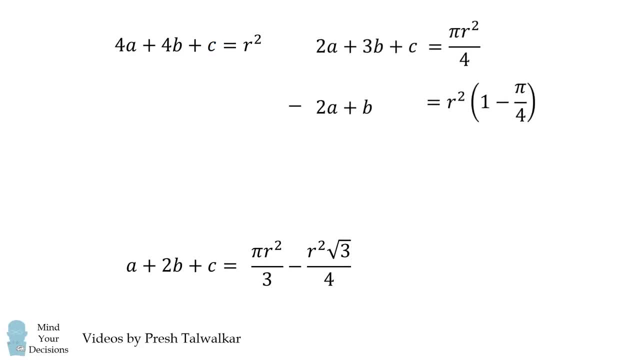 Then we'll eliminate 2a by doing the following subtraction: We end up that 2b plus c is equal to the following, which we'll substitute in to this last equation. This is an equation only in a, so we'll solve for the variable a. 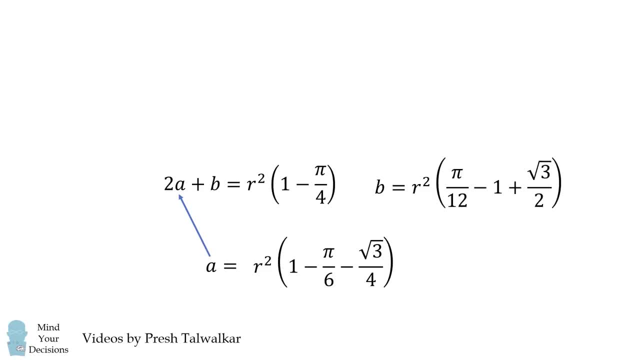 Knowing the value of a, we can substitute back and get the value of b. Knowing b, we can substitute back and get the value of c, And there you go. this is the solution to our problem. We've calculated the areas of a, b and c using only geometry and a little bit of algebra. 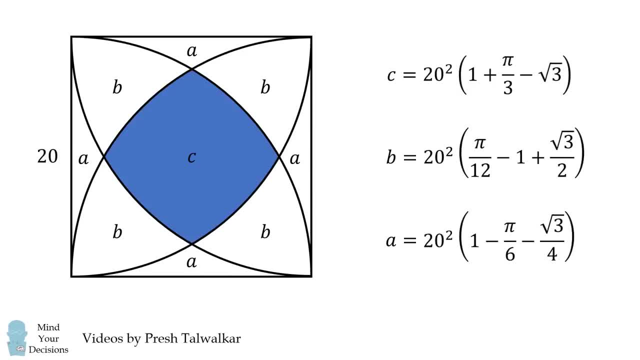 We can solve for any value of r. Suppose r is equal to 20,, this will be equal to approximately 126.06.. But I think it's awesome that we can solve for a, b and c, for any value of the side of the square. 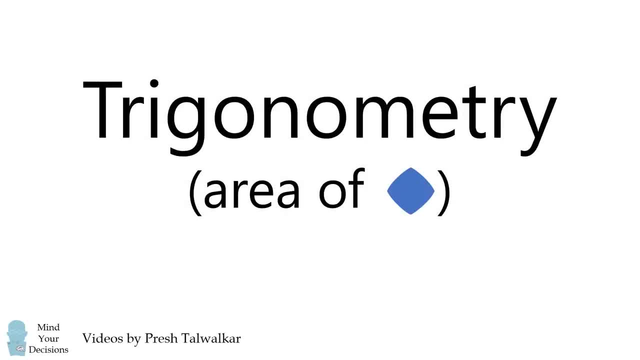 Now, just for fun, let's solve for the area of this shape using trigonometry. This is equal to the area of a sector and this is the area of a triangle. If we make this equal to a triangle in the same exact radius and the same exact central angle, 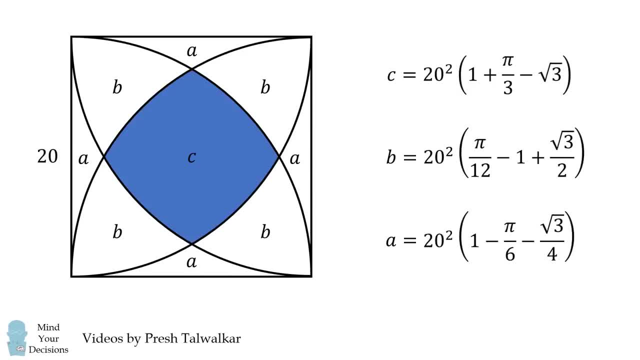 We can solve for any value of r. Suppose r is equal to 20,, this will be equal to approximately 126.06.. But I think it's awesome that we can solve for a, b and c, for any value of the side of the square. 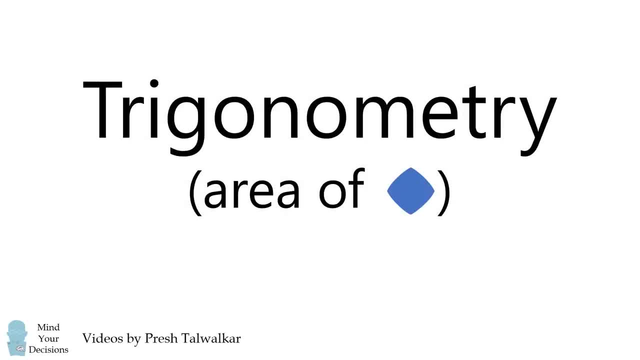 Now, just for fun, let's solve for the area of this shape using trigonometry. This is equal to the area of a sector and this is the area of a triangle. If we make this equal to a triangle in the same exact radius and the same exact central angle, 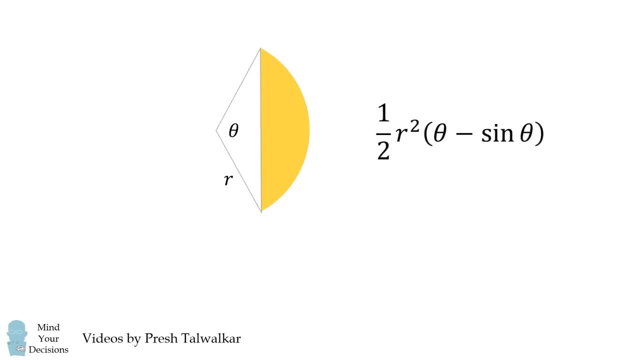 we get the area of a circular segment. Next, let's consider a triangle and use Alcashie's law of cosines. It states the following: If we make this an isosceles triangle, where both of these are equal to the radius, 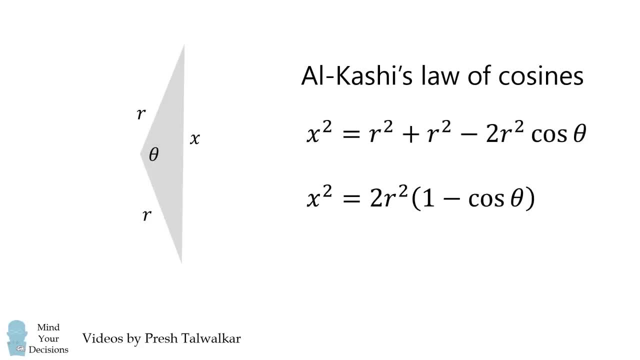 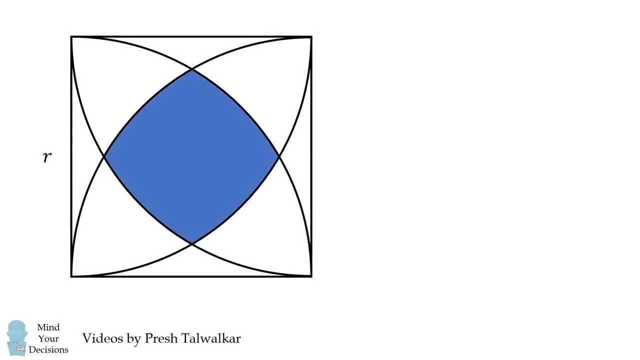 and the central angle is equal to theta, we get the following version. We'll use these formulas to solve the problem, So this shape will be equal to the following. We first will consider this radius. We have an equilateral triangle, as before, which means the remaining angle is equal to 30 degrees. 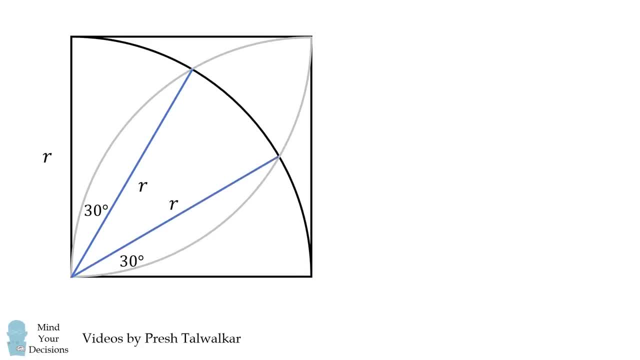 Now, if we draw this radius, that means the remaining angle will also be equal to 30 degrees, so the angle in between is equal to 30 degrees. We then calculate the area of this circular segment. We'll change the angle from degrees to radians, and then we'll use our formula. 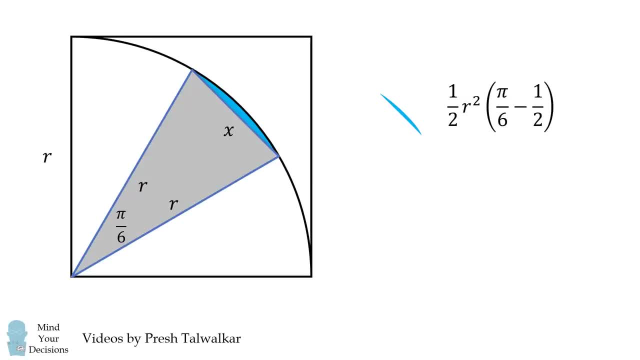 Sine of pi over 6 is equal to 1 half. We then will calculate the value of x squared using Alcashie's law of cosines. We'll substitute in and simplify. Now how does this help us? Well, if we go back to our original shape. 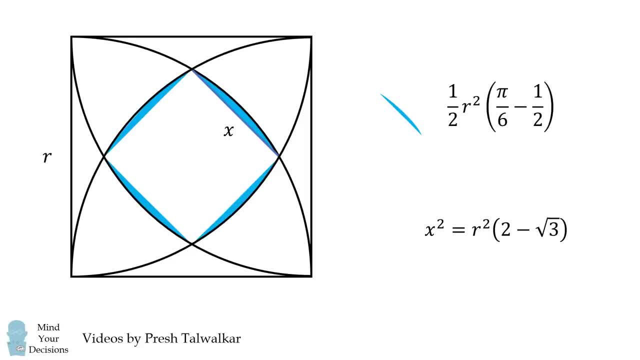 it's going to be equal to 4 of these circular segments plus the area of this square in between. So we take 4 times the circular segment and then simplify. Then we have this square with a side length of x. The area of this square will be equal to x squared, which we've already calculated. 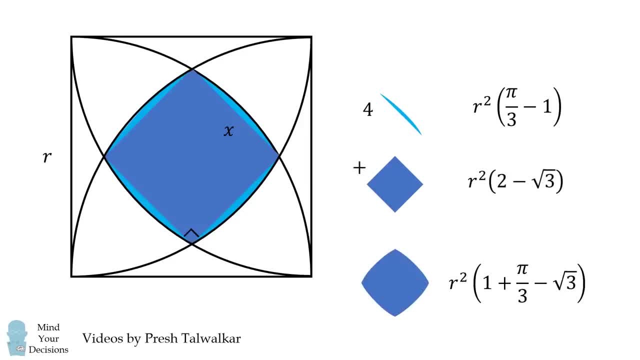 We then add up these areas and we get the area of the shape, and it's exactly the same. Let's take this, the same formula as before. What I like about this approach is that you see how the shape decomposes into other simple shapes, like a square and a circular segment. It's a great problem and I can.